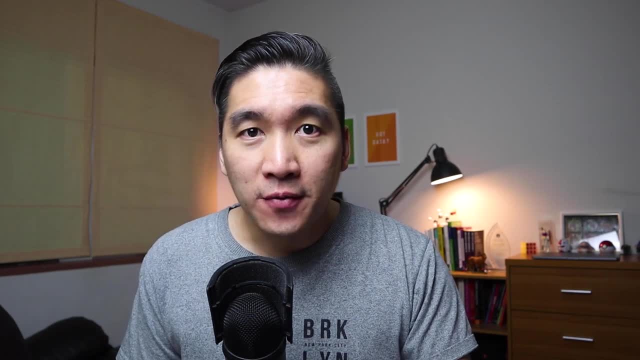 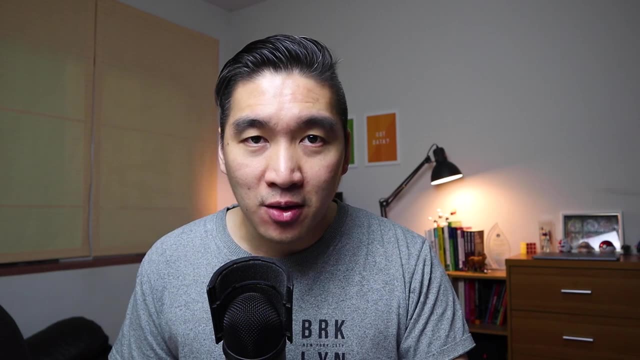 Welcome back to the Data Professor YouTube channel If you're new here. my name is Chin-Ninh Nantat Senemad and I'm an associate professor of bioinformatics. On this YouTube channel we cover about data science concepts and practical tutorials. So if you're into this type of content, 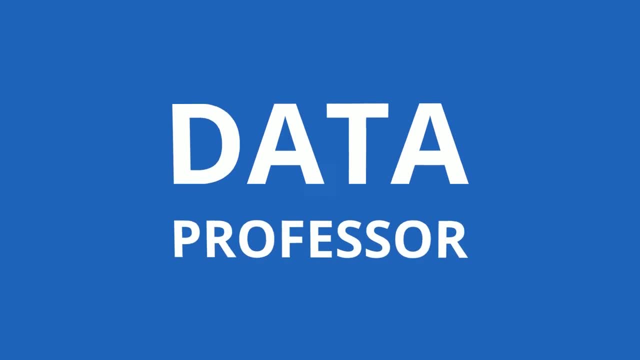 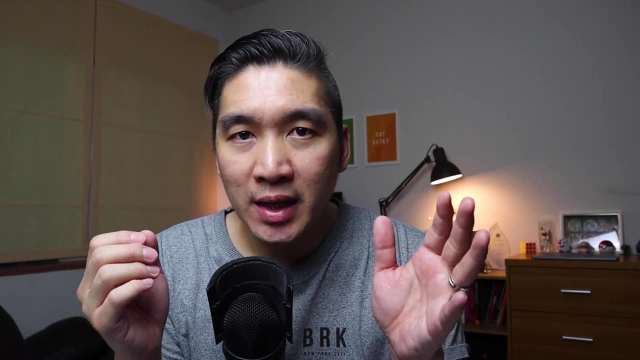 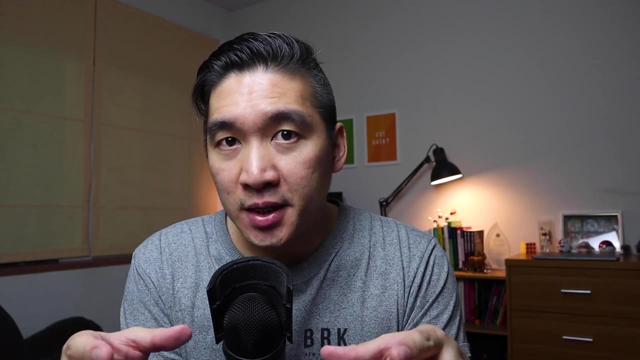 please consider subscribing. If you do data science, you know that pandas is an indispensable library that will allow you to do data wrangling, whereby you can read in your data, you could handle missing data, you could pre-process your data. It serves as the basis at which you prepare. 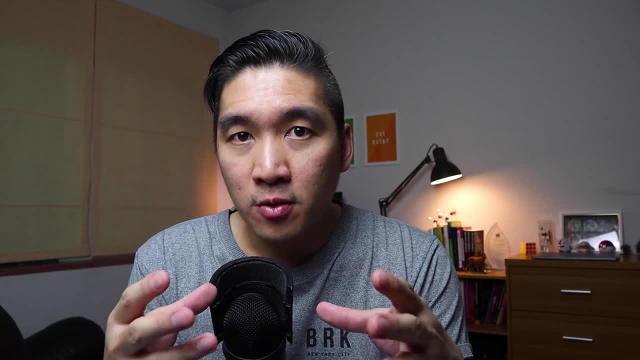 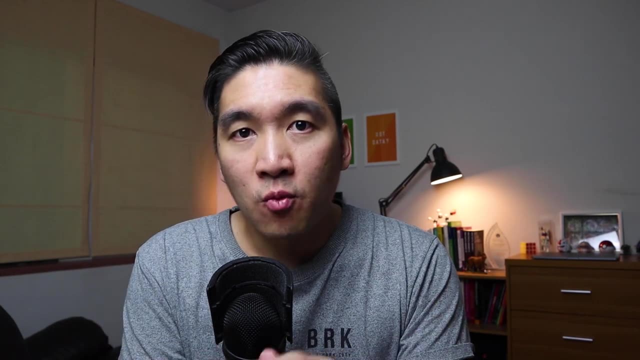 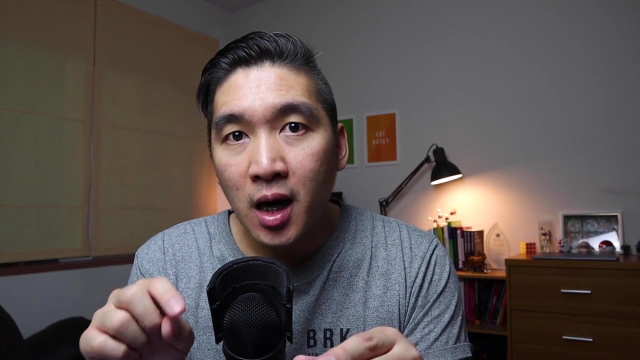 your data before it can be used for building your machine learning models, And as powerful as it can be. using it and mastering it is a great challenge, And wouldn't it be better if you could have a way whereby you could easily use the pandas library by just clicking on it? I mean literally. 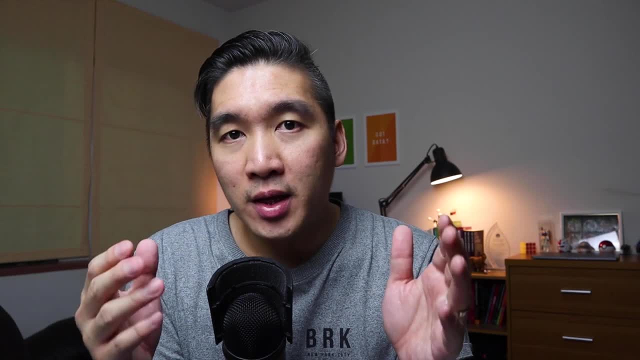 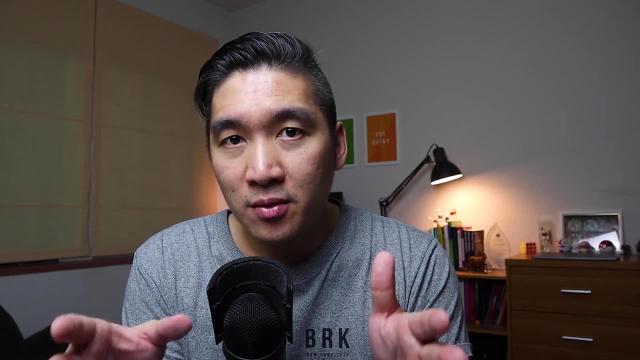 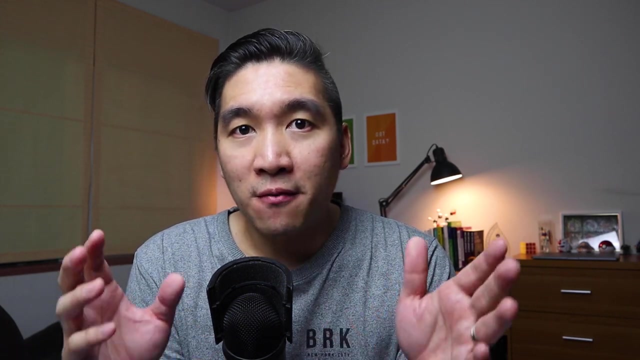 by clicking on it, And so in this video, I'm going to show you how you can use pandas by augmenting it with the ability to use a graphical user interface to easily handle the data. as if you are coding the pandas data frame but using the graphical user interface instead, And so without 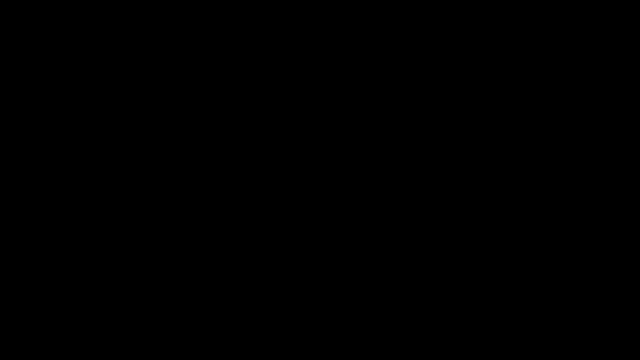 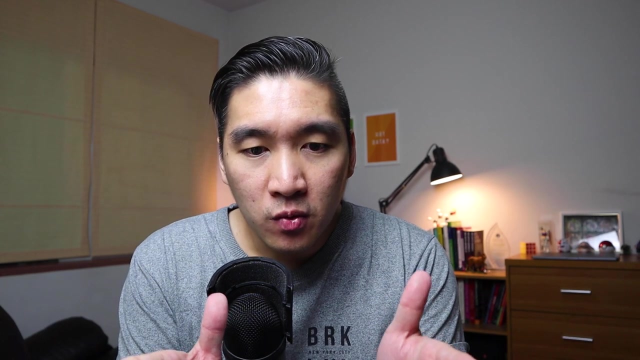 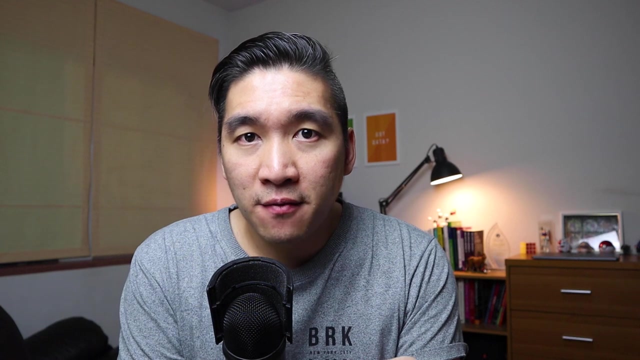 further ado, let's get started. And so the library that I'm going to cover today is called Bamboo Lib. Bamboo is in the food of pandas, And so Bamboo Lib allows you to intuitively use pandas as if it is a GUI point, and 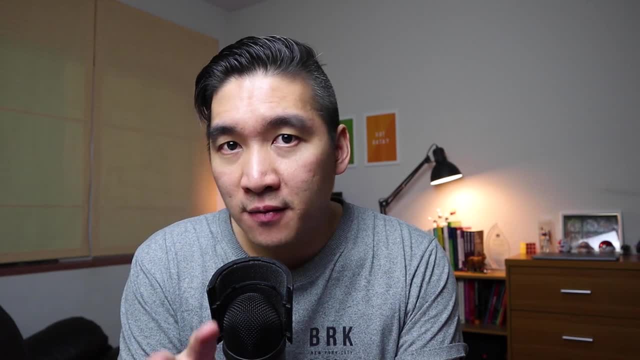 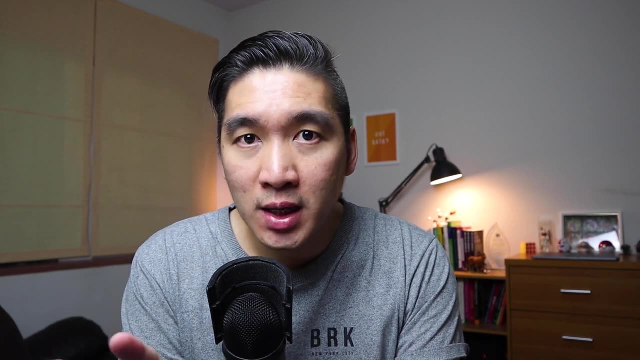 click software, And so you can essentially use all of the functionalities of pandas by easily using your mouse to help you clicking on the options that you want. So this is the website of Bamboo Lib, And if you would like to have a look at this website, you can just Google for it. 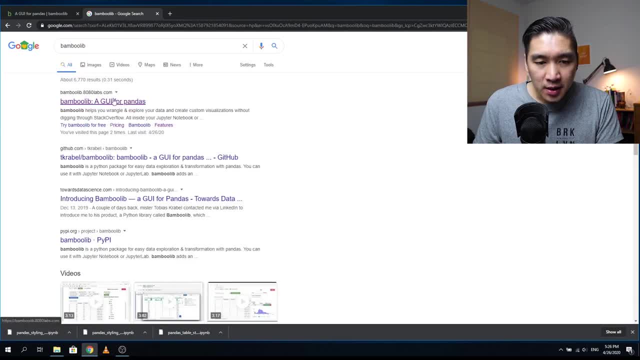 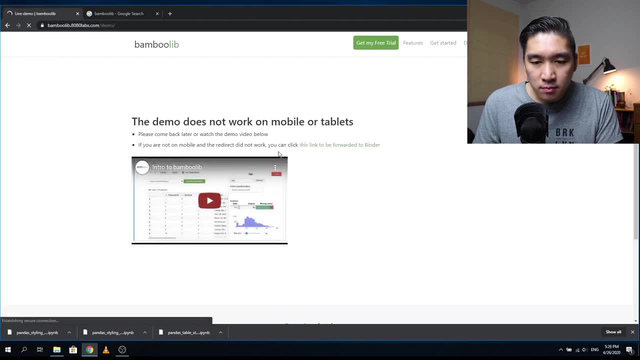 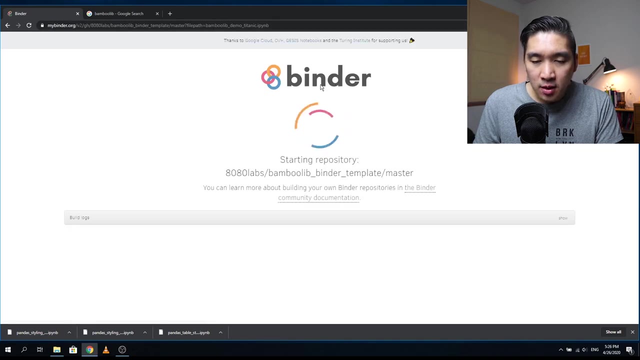 Just type in Bamboo Lib And then it's going to be the first link, And so you can click on the Try Live Demo, And then this will create an interactive notebook using Binder. Wait just a moment. So while we're waiting, let's have a look at the web again. So before we continue further, 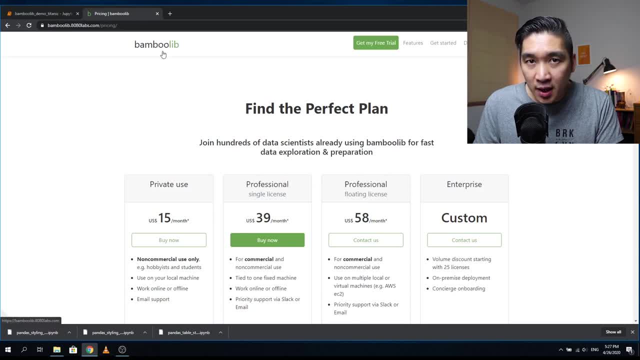 let me make a note that Bamboo Lib is for a fee, meaning that you have to pay to use this, And so they have four plans for you to choose from: $15,, $39,, $58, and also custom, And so $15 is. 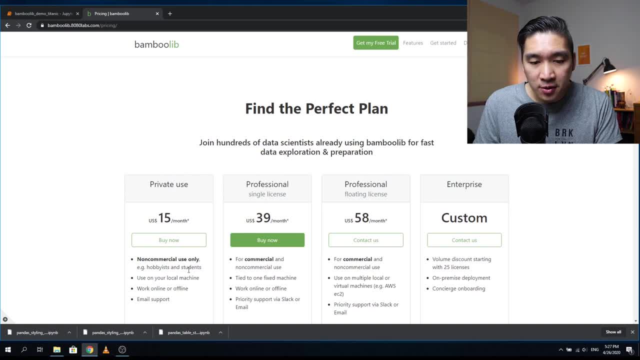 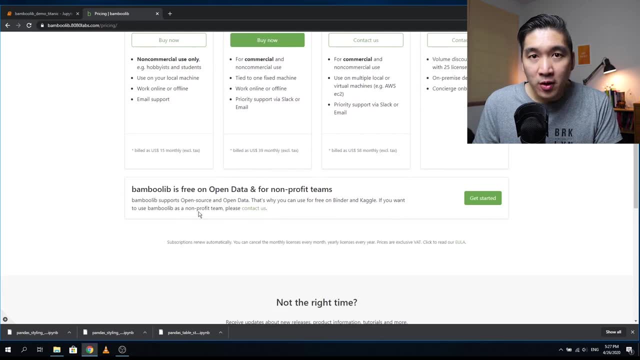 for the private use, So it's for the non-commercial user, And so this is particularly suitable if you want to use it for your private data. However, if you would like to play around with the Bamboo Lib and use it on open data and nonprofit teams, you can also use Binder and Kaggle. So let me show you. 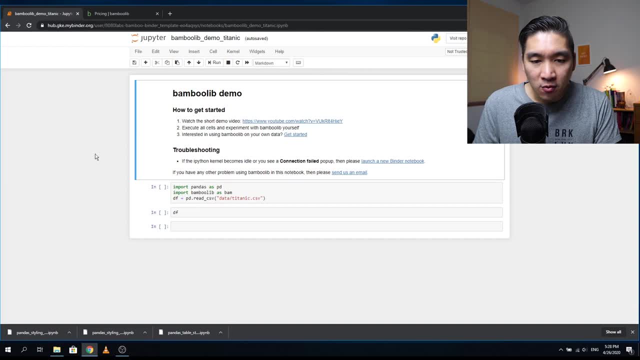 how you can use Bamboo Lib on Binder. So let's head over back to this notebook And so let's have a look, And so here is just a couple of lines. The first line of code here is: import pandas as PD and then import Bamboo Lib as BAM, And actually you could also replace this. 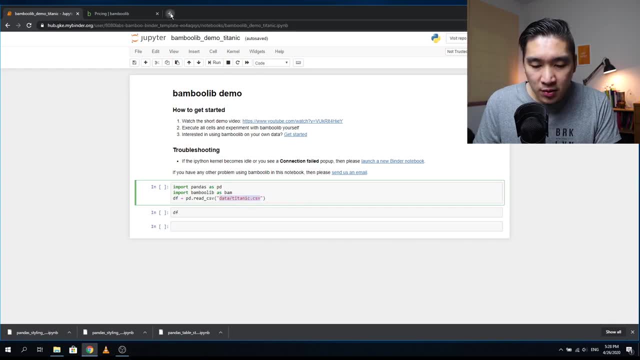 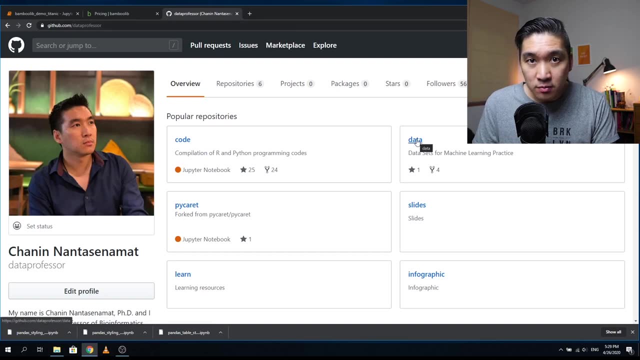 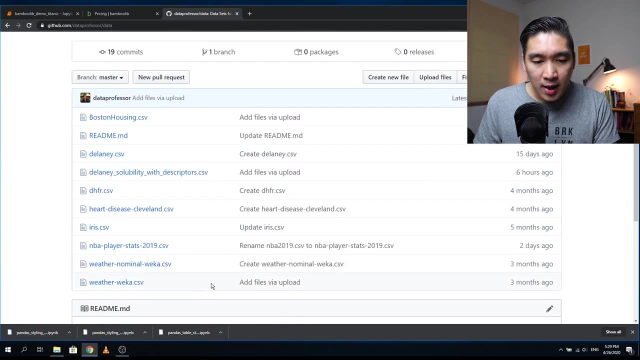 with a data set of your choice. So let me show you. Let me use the NBA player stats that we have performed web scraping in a previous video, So links in the description and also up here. Okay, so let's click on data And click on the NBA player stats 2019.. Click on raw. 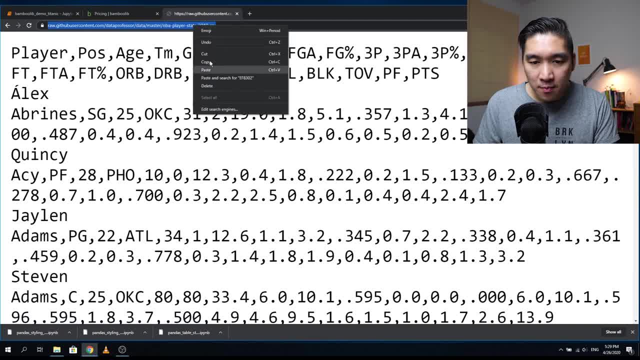 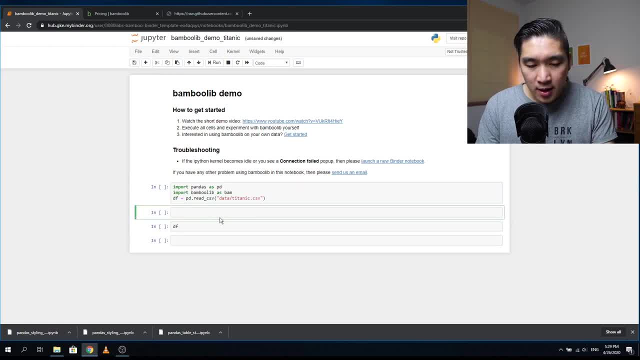 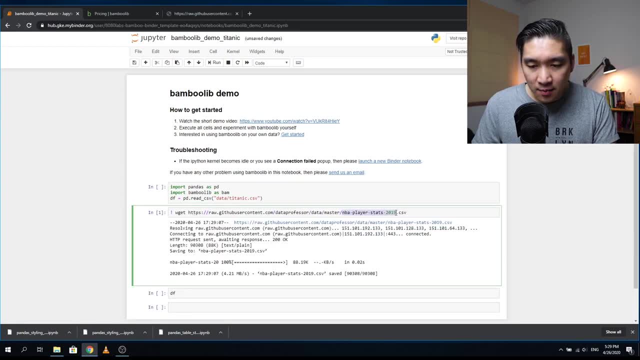 And then click on the URL, copy it. And let's insert a code cell here and type in exclamation mark W- get, and then paste the URL. Okay, load the file and then copy the name of the CSV, put it here. 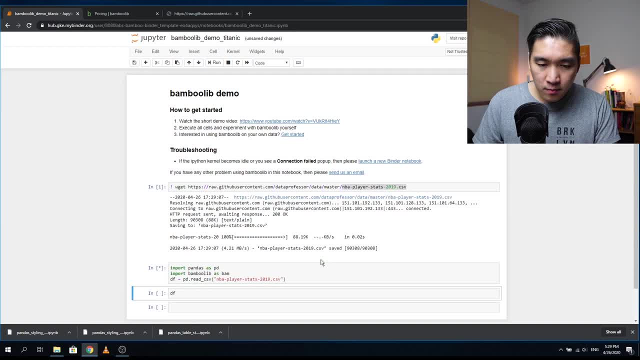 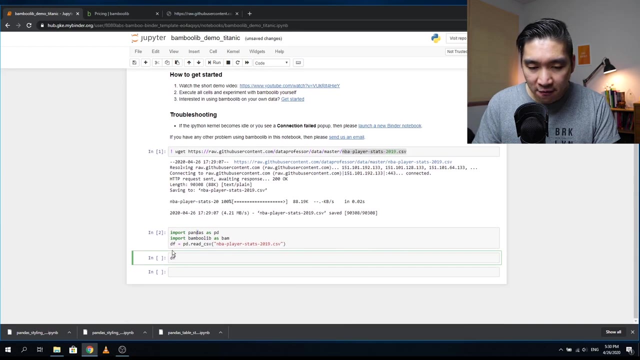 Let's move this down, Okay. so here we're going to import pandas as PD and we're going to import bamboo lib as BAM, And then we're going to use pandas to read in the CSV and assign it to the DF variable. And let's have a look at the F And you want to click on the show: bamboo lib UI. Okay, 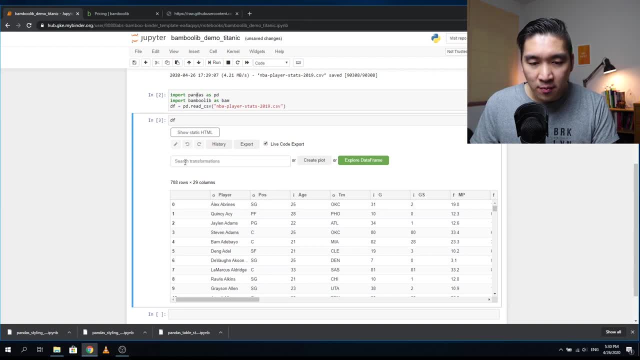 and so here you have three options: you want to search for the transformation that you want to perform on the table, or you want to create a plot, or you want to explore the data frame. So let's start from the right and then we'll move our way to the left. So let's explore the data. 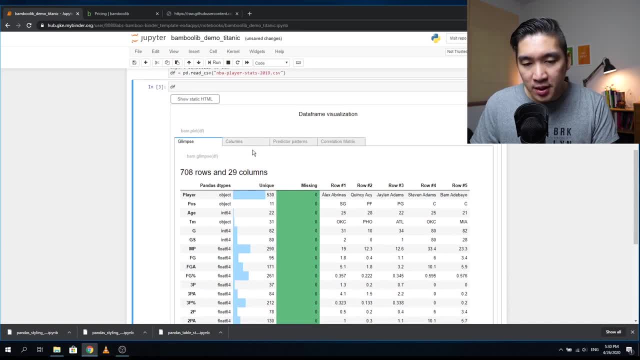 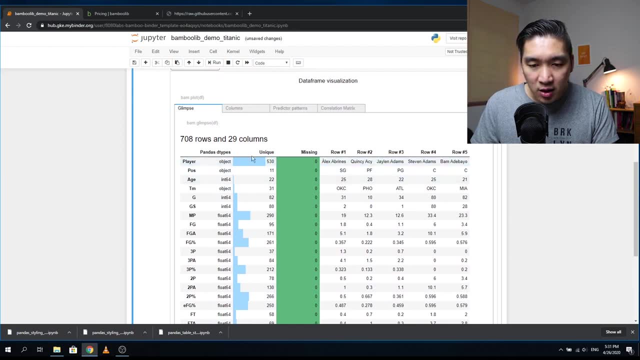 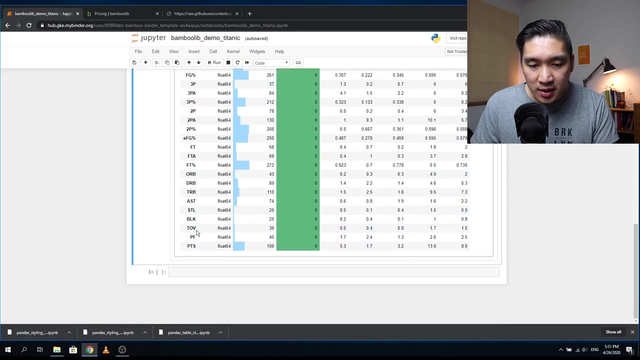 frame. Okay, so notice that this might resemble pandas profiling a little bit. So this first tab will provide you a glimpse of the overview of the columns. So here you're going to see the name of the columns: player position, age, team games. okay, and set to run to points. column: 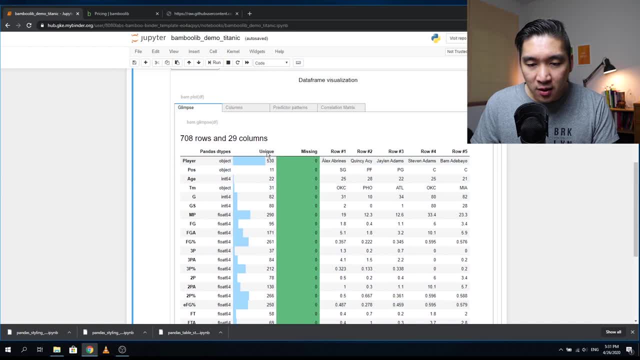 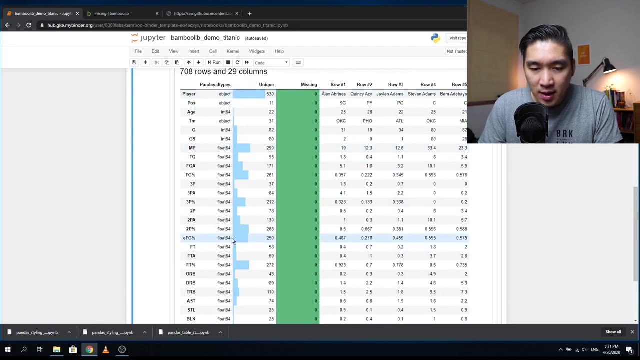 And for here you're going to see the number of unique values. So you're going to see that out of 708 rows, there are 530 unique player values, And so you're going to see that the player name has the most unique value, followed by the MP column and 2p percent and the EFG percent. Okay, so this 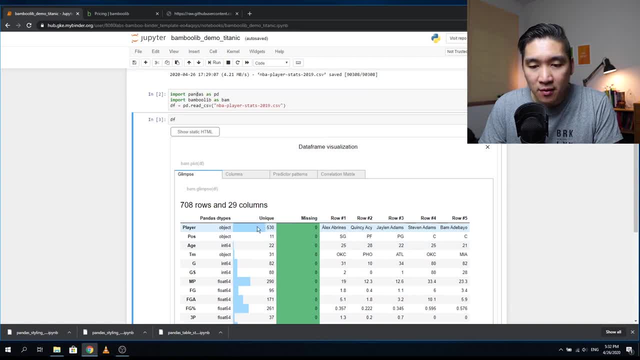 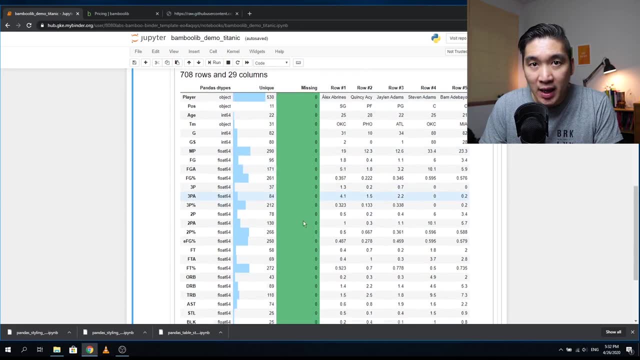 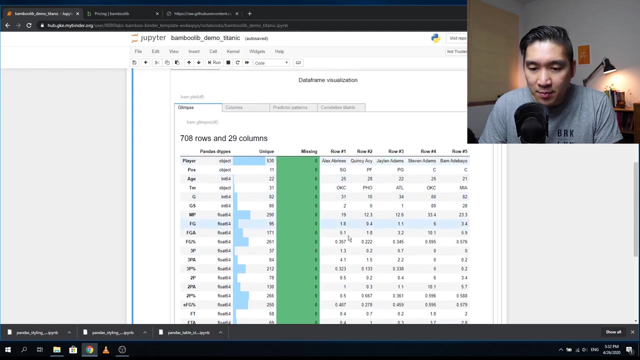 will just tell you the relative uniqueness of the value of your column, And so it's also good to be able to view the number of the missing values at a glance here very quickly, And here we see that there's no missing value. And then these are just the examples of the first five rows. 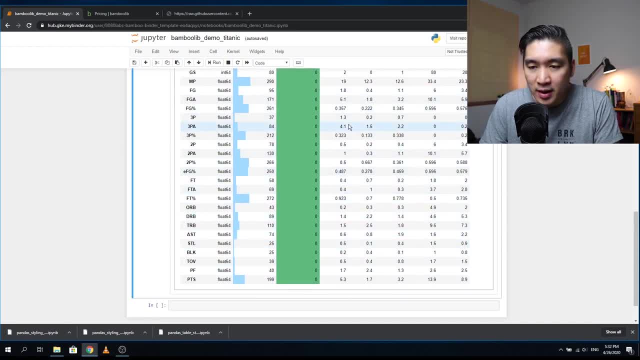 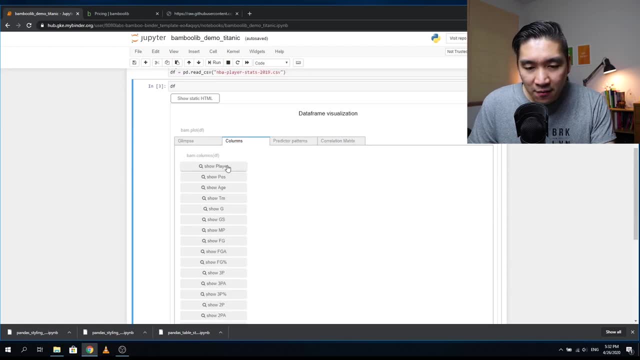 Just to give you an overview of what values are in the columns of the roles here, And let's click on the second tab column And then you could dive in into each of the columns. So let's start from the player right And then you're gonna see, okay, which one has the most. 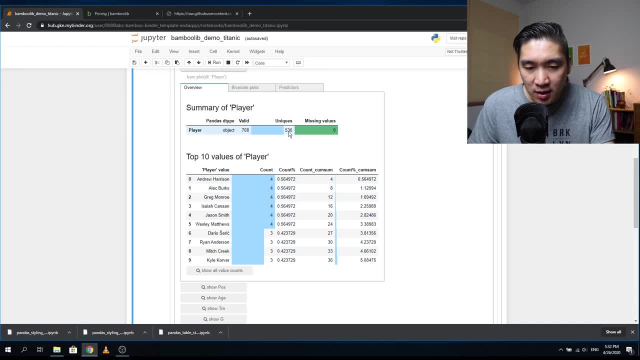 right. Like we know that there are 530 unique names, And for the 530 unique names, some names are found more than one time, And so, for example, Andrew Harrison is found for four times, Alec Burke is found for four times, And probably they were traded to another team during the season. 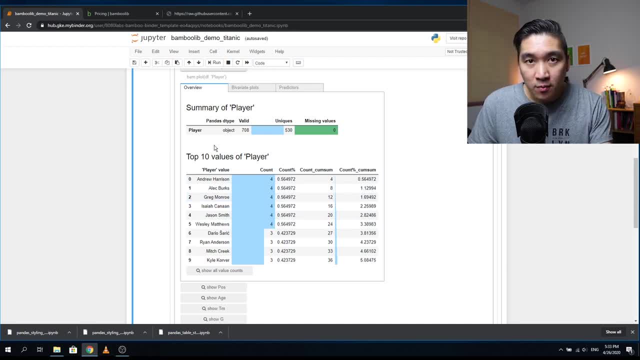 So if you might be interested in the trading of players from one team to the other, etc. you can have a look at this as well, Like, for example, which was the most traded player. Okay, you could click on the following column: show position, or we can even hide the player here. 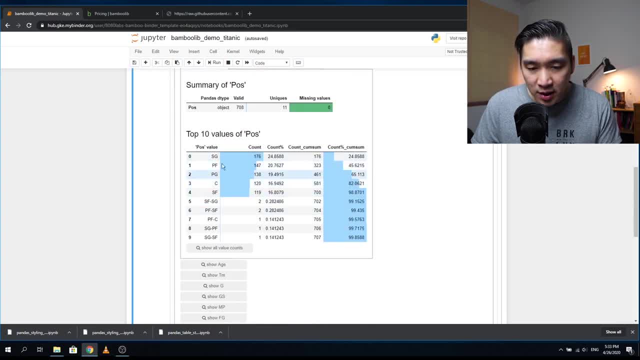 Okay, and so you see the traditional positions are shown in the most populated here: shooting guard, power forward. point guard center, small forward. okay, and you see the relative distribution. out of the entire data set, shooting guard accounted for the most, at 24%. 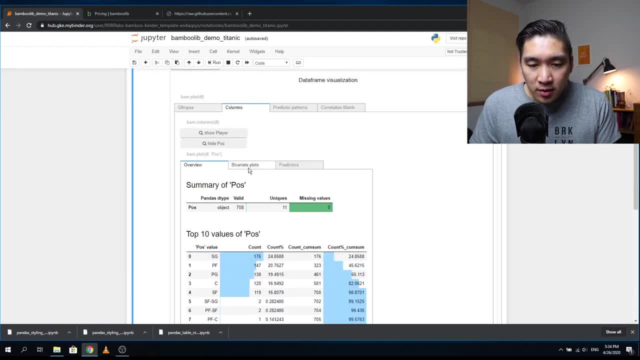 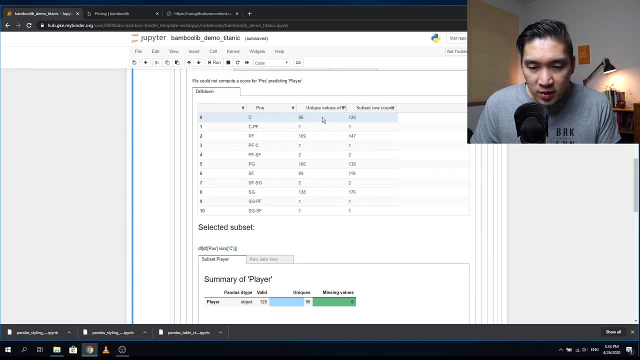 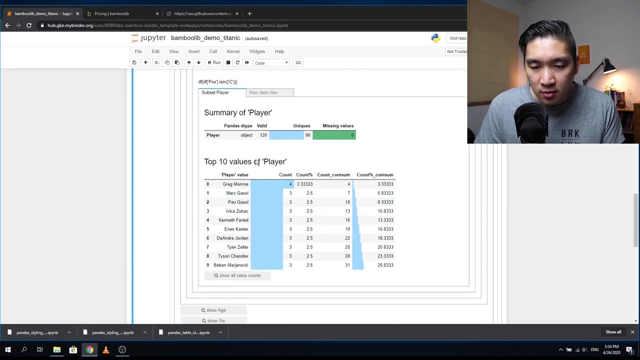 right, followed by power forward. okay, And you can also have a look at bivariate plots. For the center, there are 96 unique values and there are 120 roles, top 10 value of players. So here you see, all of these players are center, having the position of center, And so, as you, 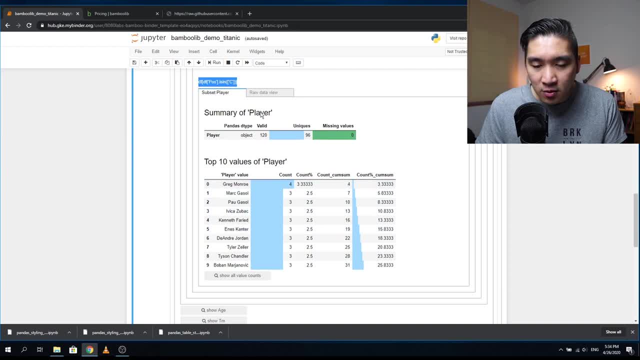 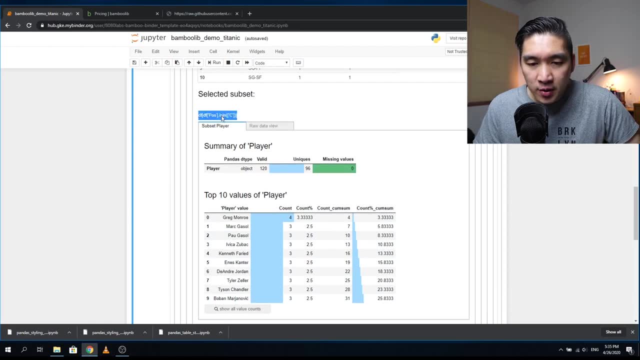 notice here, it will automatically use this command in order to give you this view. So for those of you starting out pandas, please also make note of what command are shown here, So you could just copy this and then implement it in your code as well, And then you can also have a look at. 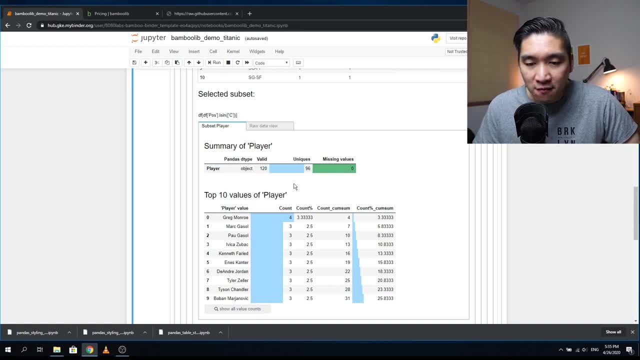 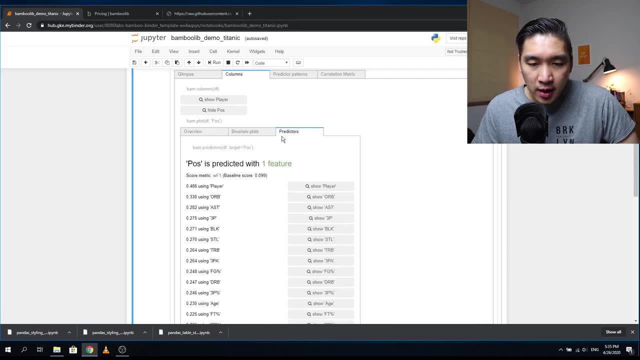 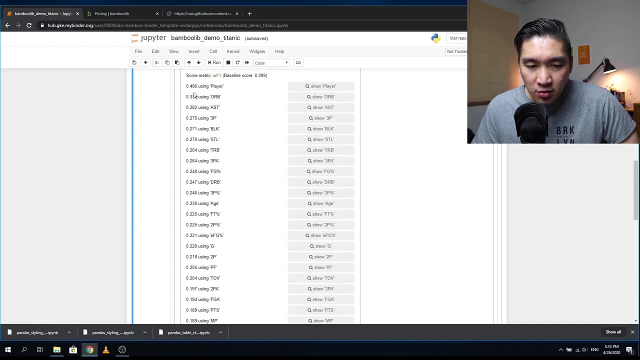 So you can learn along while using this interactive pandas bamboo lib library, So you could also make use of it as a learning tool. Okay, and it has this predictor function where position is predicted with one feature and it shows the relative score metric. So, probably coming from the 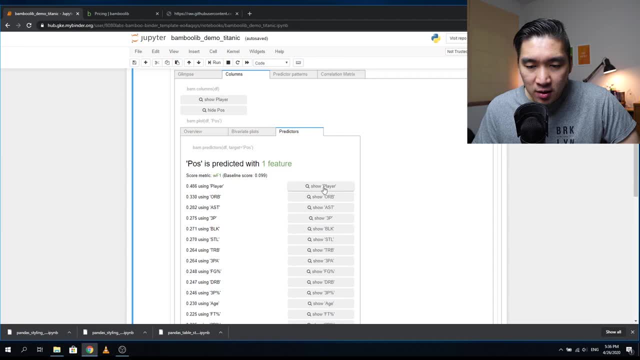 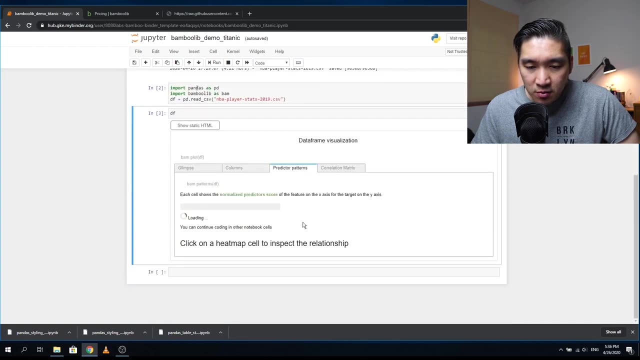 Pearson's correlation coefficient. it might be interesting to have a look. So this is very nice. it allows you to play around with the data, eyeball the data. So it's good when you're starting out in your analysis and you don't know the data set yet or you want to gain an. 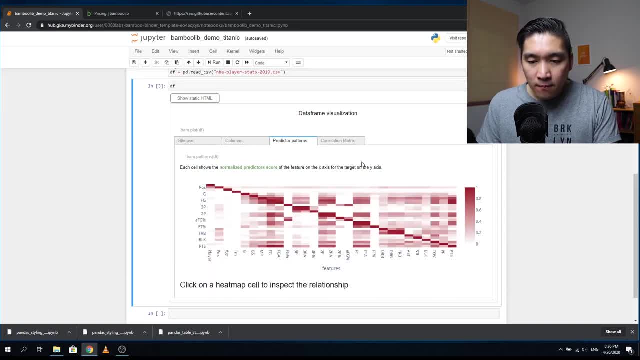 understanding of the data set. So you could just click, click, click, Because sometimes when you're starting out on the data set, you might not know which type of exploratory data analysis plot that you want to use. So in most of the cases you might be using all possible plots and graphs And so 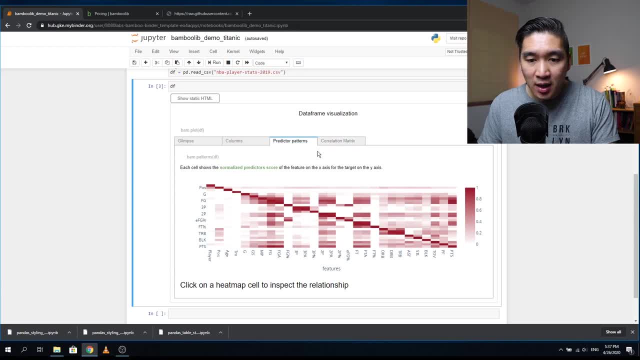 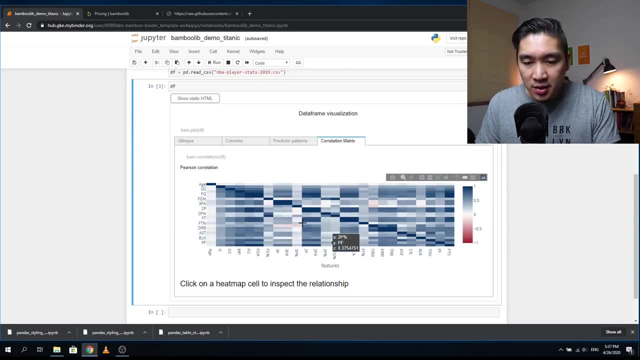 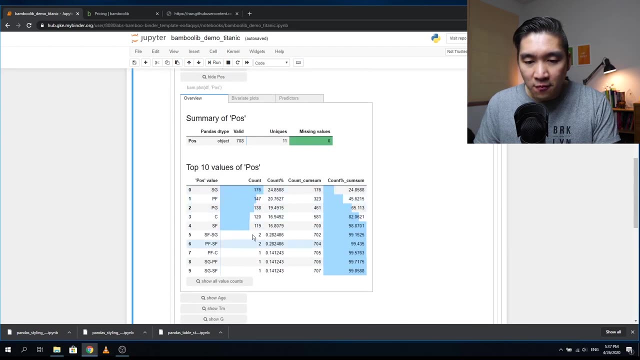 this pandas bamboo lib comes in handy. it allows you to just interactively click and drill down through the data frame And looking at various correlations or various plots, various columns right, various bivariate plots, or having a look at the overview of the data set. Okay, so let's. 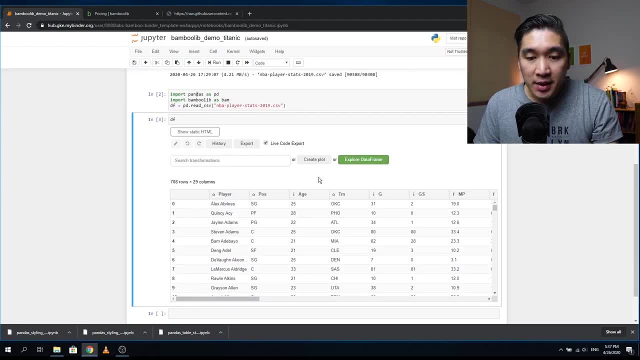 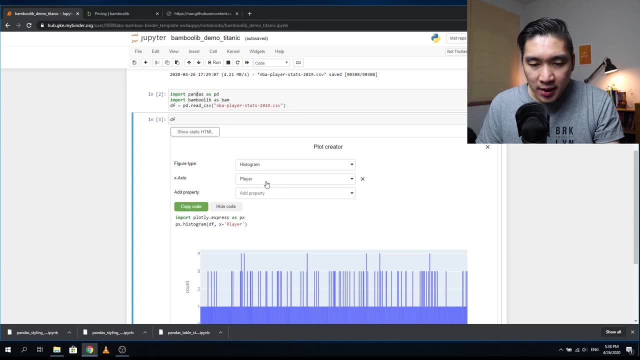 close this. this is the Explorer data frame. Okay, and so let's continue with the create plot, And so here you could select histogram: say that you want to use the x axis to be the player name, and let's add y axis. 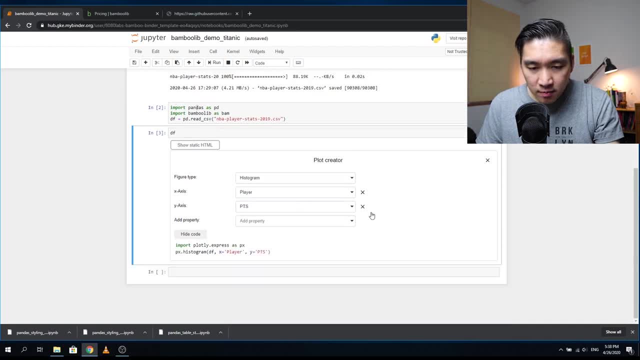 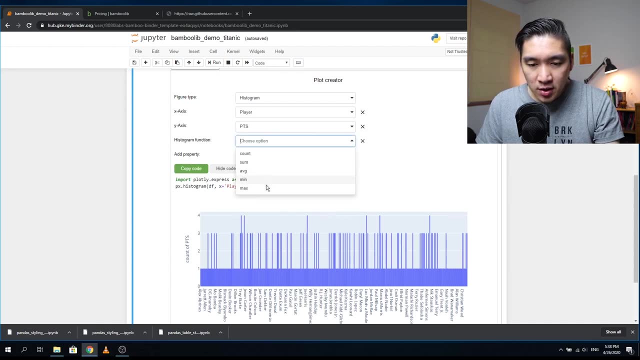 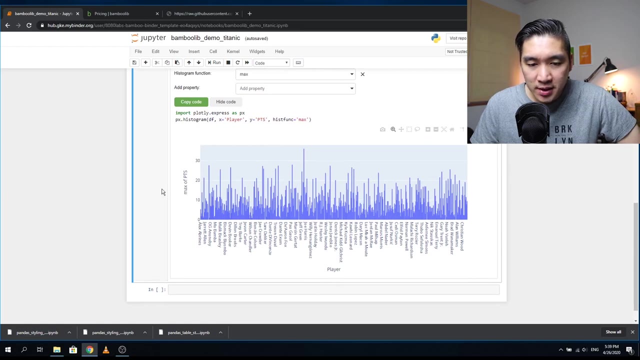 and then the y axis. we're going to select points And add property. here we're going to use the histogram function And we're going to show the maximum, And so this gives you a relative overview of which player scores the most points, And you could just hover the mouse over it And 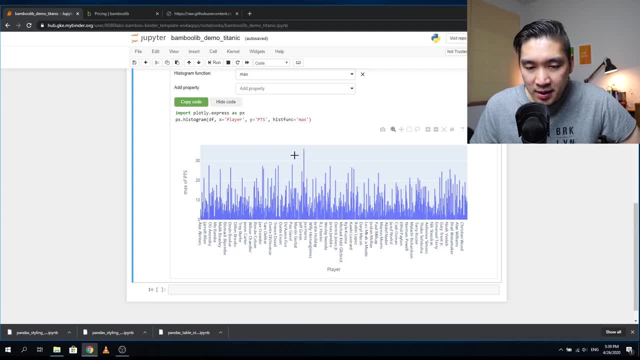 then you see that, okay, it's James Harden here. So you make note that it's kind of like the bars here are spikes And you could set like a threshold here, like, okay, anyone exceeding 30 points, and you see only one value and you see James Harden, and let's say that between 20 and 30,. 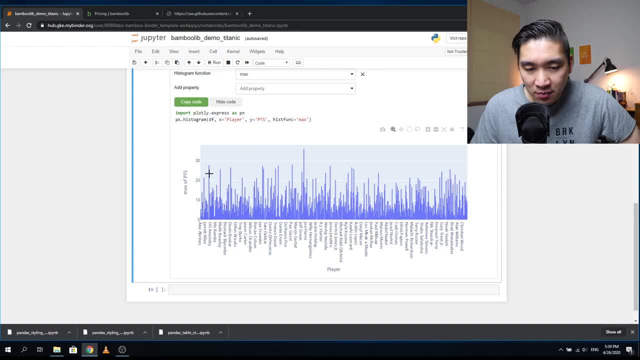 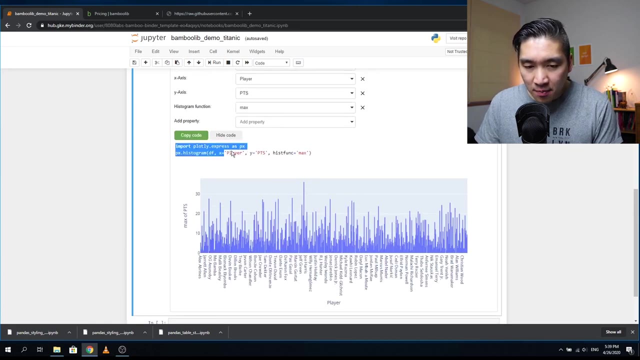 and you just move your mouse over from left to right and see what names comes up: right, 27.7,, 25.6, right, just interactively, you know, just playing around eyeballing the data. And let's say that you would like to create this plot, you could just copy it or copy code, right? 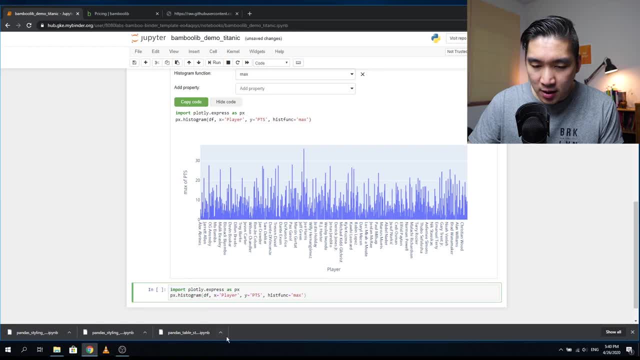 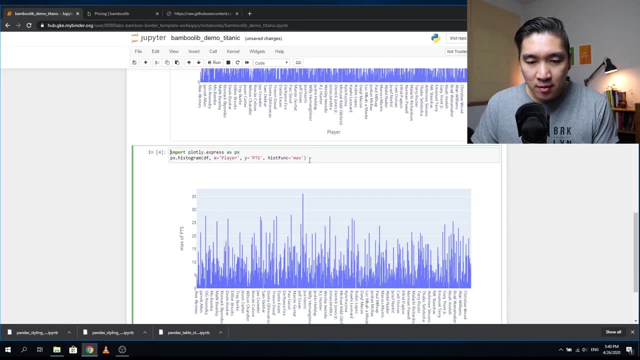 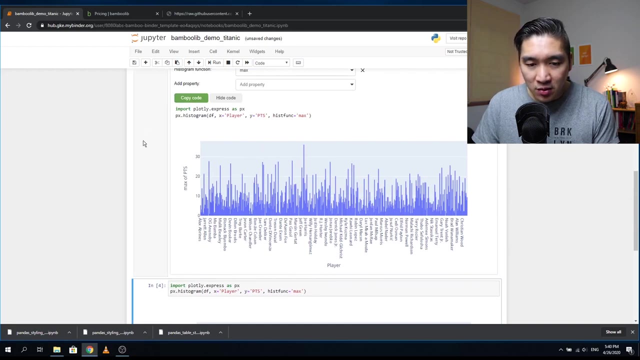 to copy the code already, And then you just paste it down here and then run the code cell And so you get the exact same plot as shown here. So it comes in handy when you're eyeballing it and then you see a particular plot that you like, So you could just copy the code and paste it down. 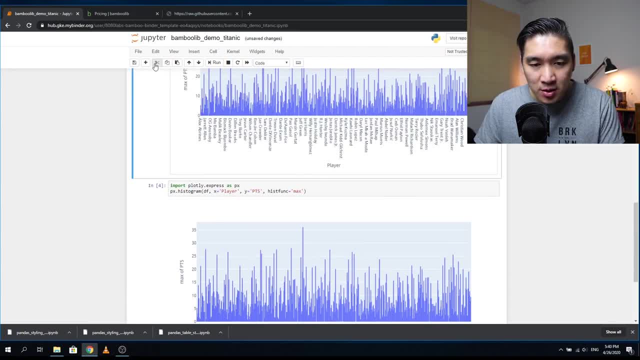 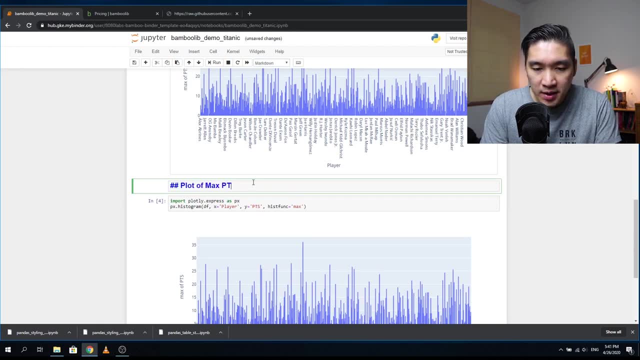 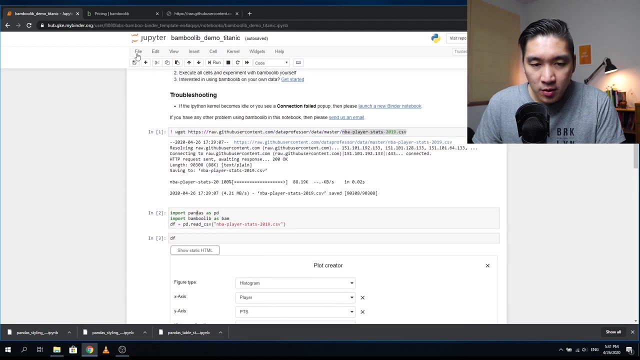 here, Right? And then you could also annotate this a bit in order to add meaning to it. A lot of max points versus player, Okay, and so with this notebook, you could also save it, right? you can save it as a PDF. 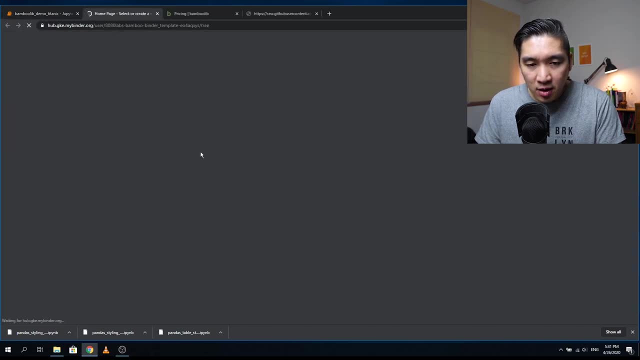 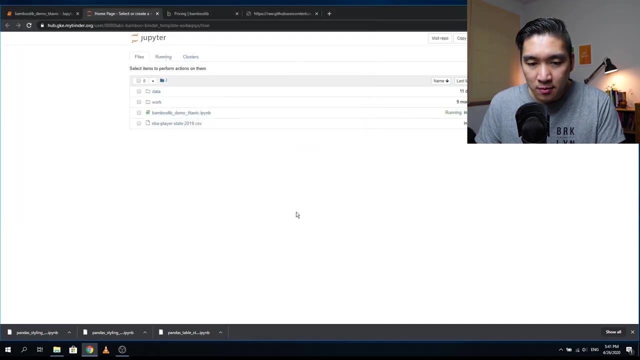 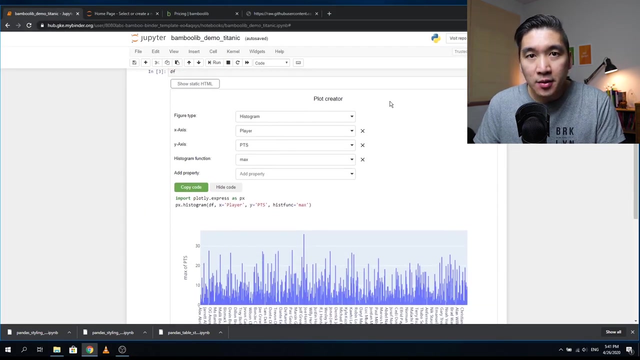 you can save it as a notebook file as well, And the good thing is, you can also open it up. You could upload your own data in here, Right, and then perform your own custom analysis as well. Okay, so let's close the plot, And so you could play around with the different types of plots. 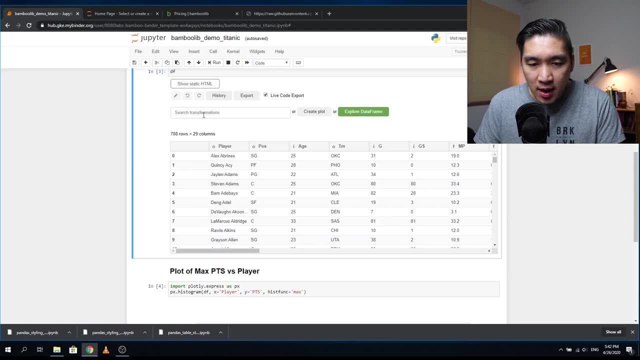 here, And so let's move on to the next one and search transformation. So here you could do various sorts of things that pandas allows you to do, like filtering, sorting group by aggregate data, join, merge data frame, replace value, string manipulation. 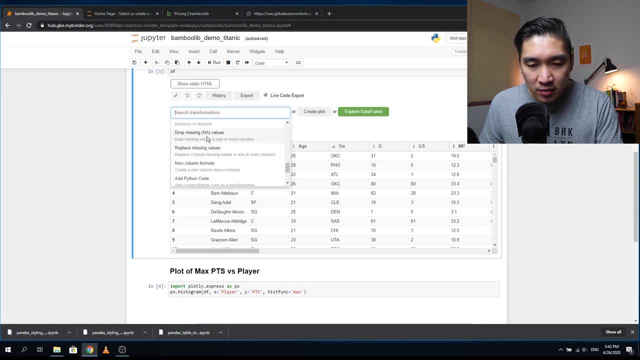 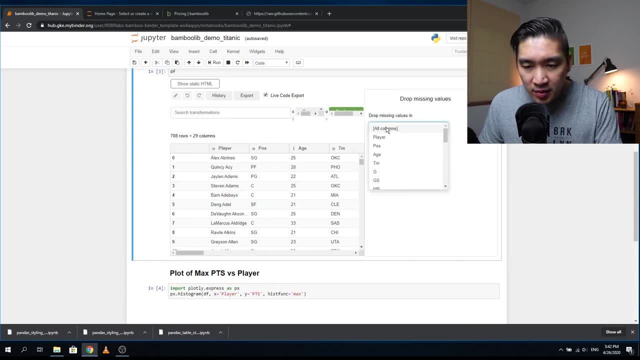 bin columns, pivot the data, drop missing values or even replace missing values. Let's click on drop missing value and then drop missing values in all columns, And then the name of the new data frame. let's just maintain it at the same name. 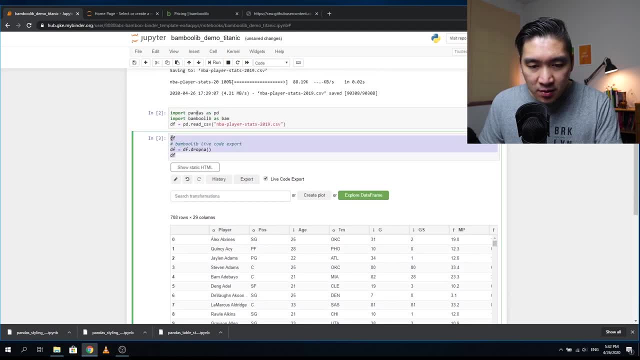 execute, And then you see that it also gives you this block of code here. So it's good for the newbie, it's good for the beginner And so you can learn along, as I have mentioned previously. And so if you want to remove missing value, then you know, okay, that it is the drop any function. 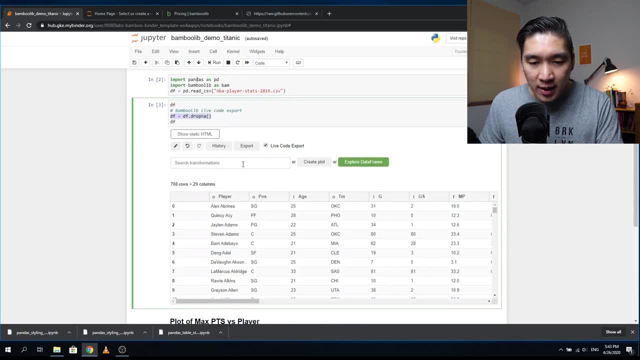 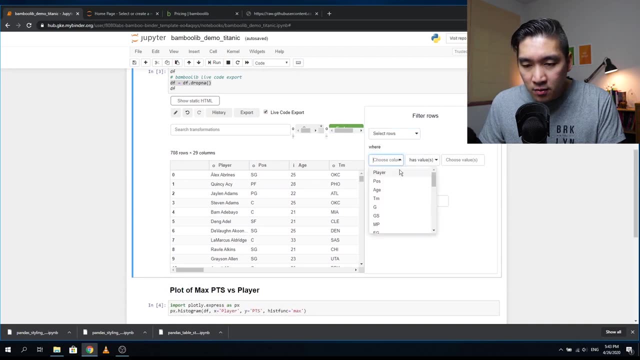 okay if you're starting out okay. so this comes in very handy. And let's see, you want to perform some other, let's see filtering, and then you want to select roles based on some condition. So let's say that you want to show players having points greater than 20.. 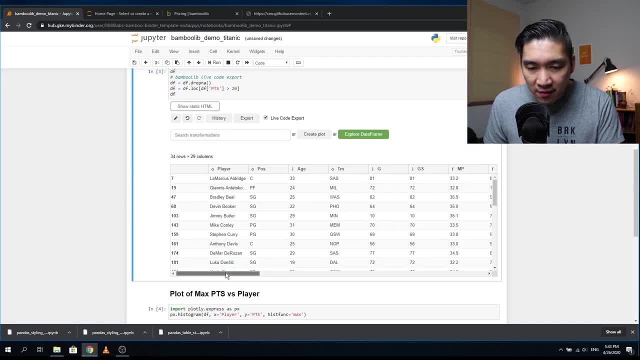 Execute And then you're going to see only those having points greater than 20.. Right, And then you see the name here and you see that there are 34 rows by 29 columns. So you see that there are 34 players having points greater than 20.. 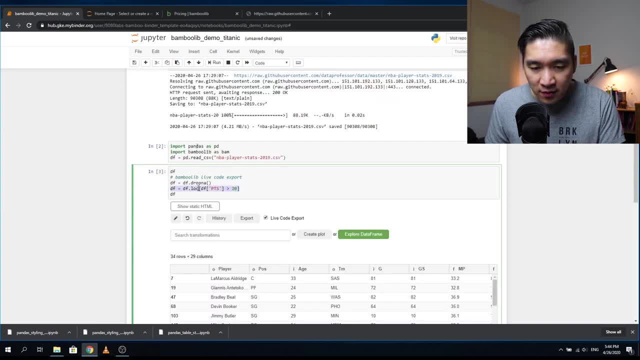 Make note that this is the code that was used to filter the data. Okay, and so we have done something similar in a previous video on exploratory data analysis using pandas, And so, as you will see, this very easy: you just click on it interactively, Select roles or even. 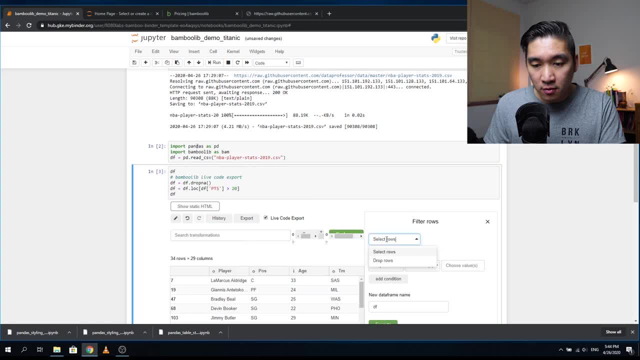 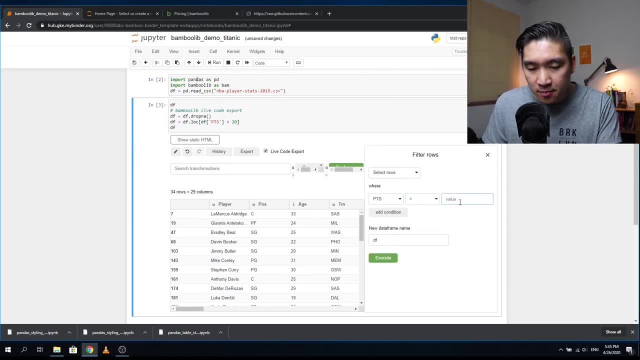 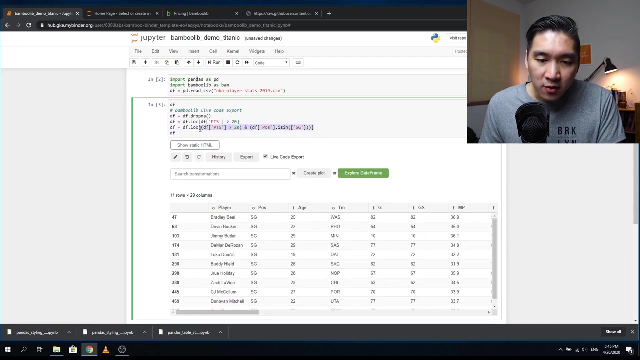 want players having more than 20 points a game, And let's add another condition, And you want only the shooting guard. Okay, so you want players having more than 20 points and their position is equal to shooting guard and then execute, right, And so it's going to run this block of. 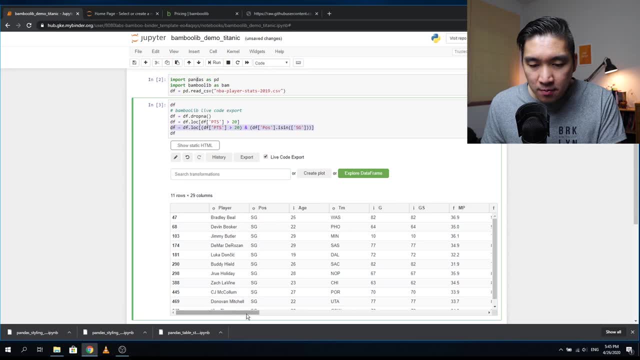 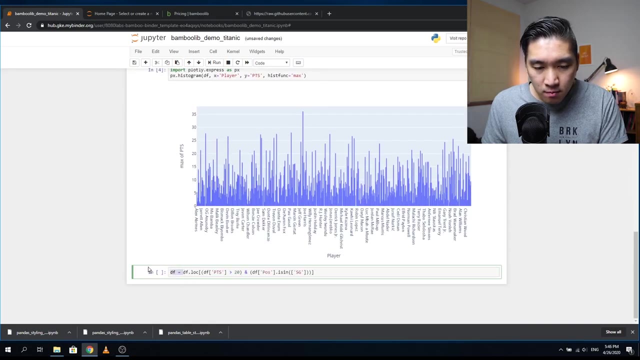 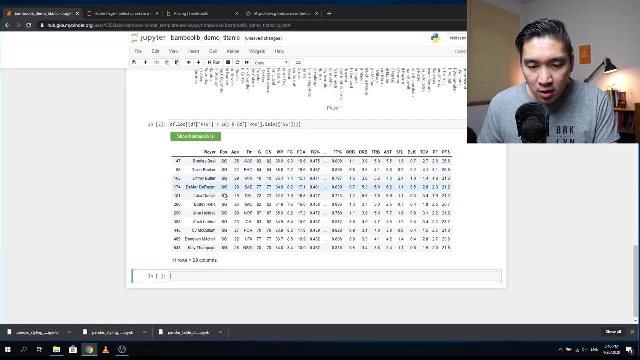 code here, And so all of these are shooting guards, Okay, having more than 20 points. And you could also copy this particular code And then show it here. Right same data, Okay, Only shooting guard, more than 20 points. Okay, so the possibility are endless and you are able to.